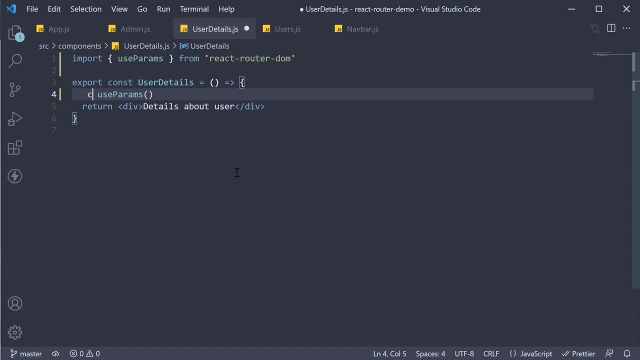 of key-value pairs. Let's call it params. So const params is equal to use params. This project contains key-value pairs of the dynamic params from the current URL. The parameter we want to access is user ID. Let's store that in a constant. 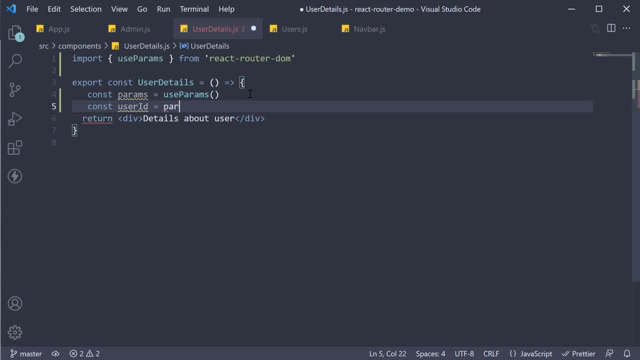 const. userId is equal to paramsuserId. It is important to note here that userId on the params object corresponds to the dynamic segment we have specified in the route. It is more important to note here that the userId on the params object corresponds to the dynamic segment we have specified in the route. 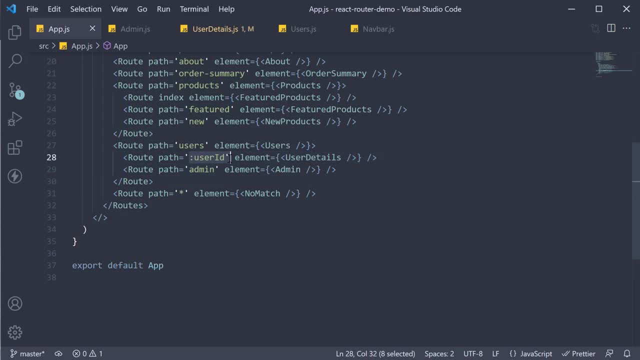 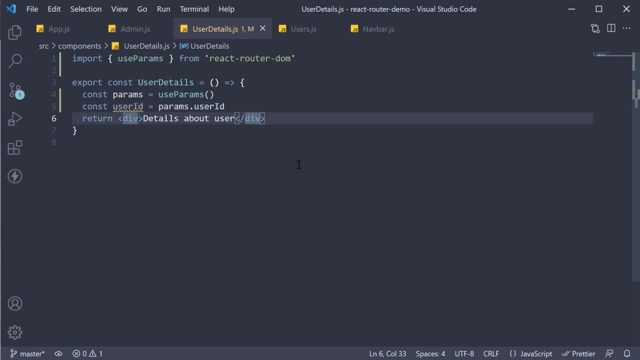 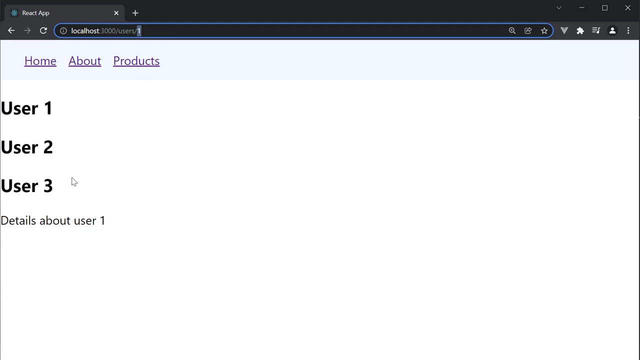 So params, or the dynamic segment, becomes the constant constant in the route config, colon- user ID. once we have the user ID, we can render it as part of the JSX details about user and we render the user ID. if we now save the file and head back to the browser, navigate to slash users, slash one and we see the text. 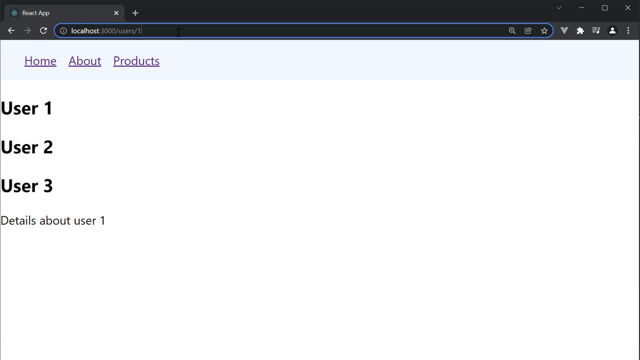 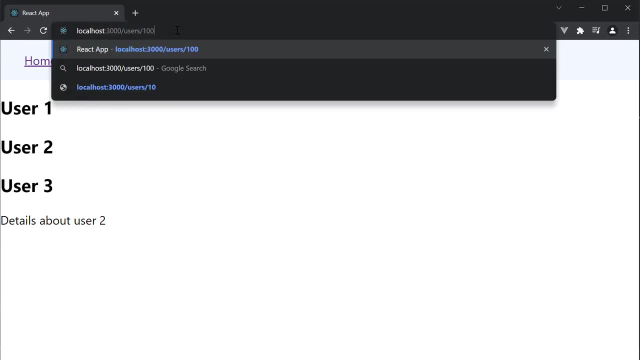 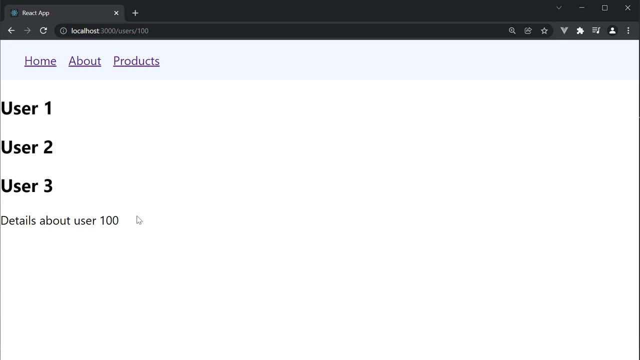 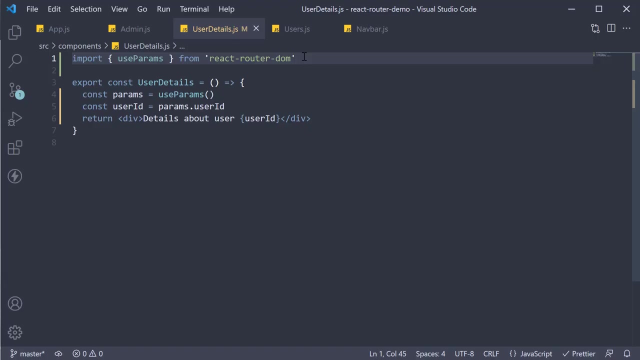 details about user 1. change it to slash 2. you see details about user 2. slash 100. details about user 100. so this is pretty much how you get hold of URL params in your component: import the use params hook and invoke it and access the. 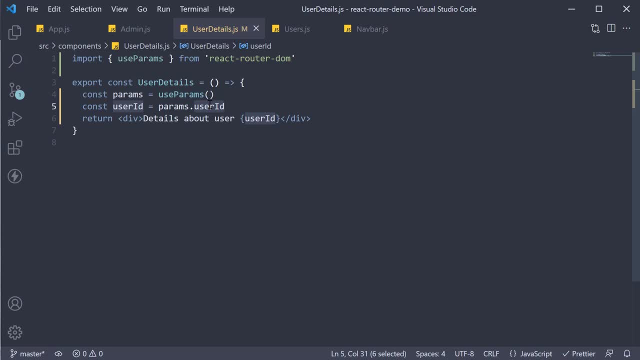 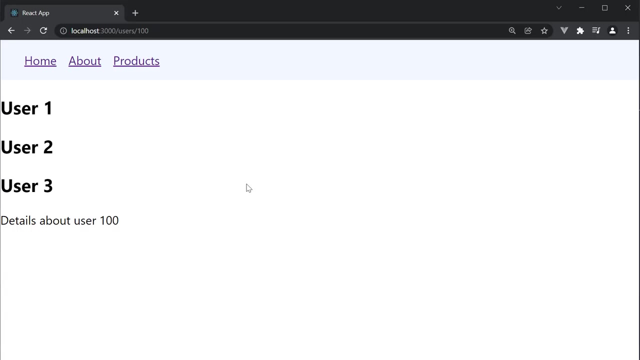 property on the returned object. if you wish to, you can destructure user ID in the same line. so const the structure user ID and delete the next line. save the file and the output remains the same. in the next video, let's take a look at search params with react. 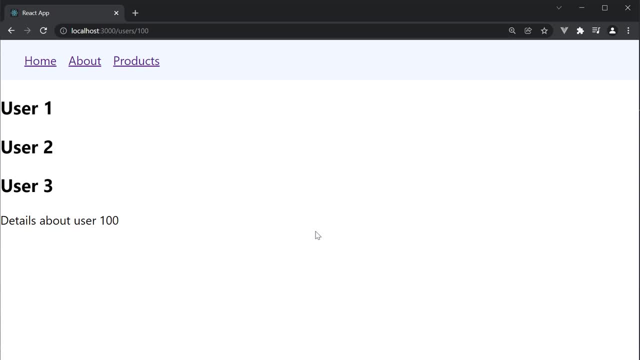 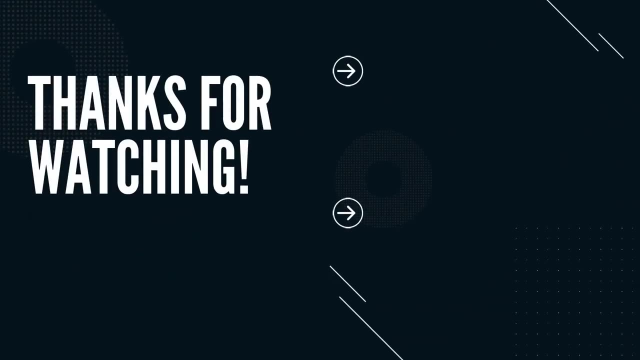 router. thank you for watching. please do consider subscribing to the channel and I'll see you in the next one. you 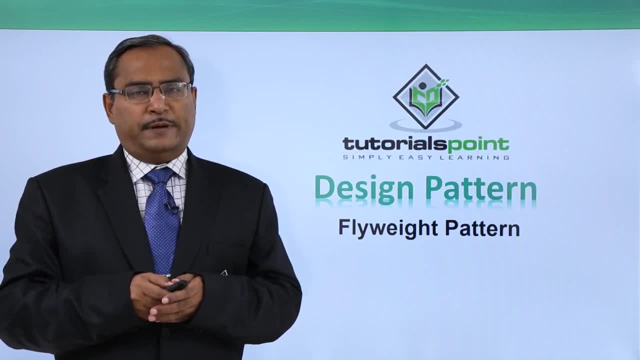 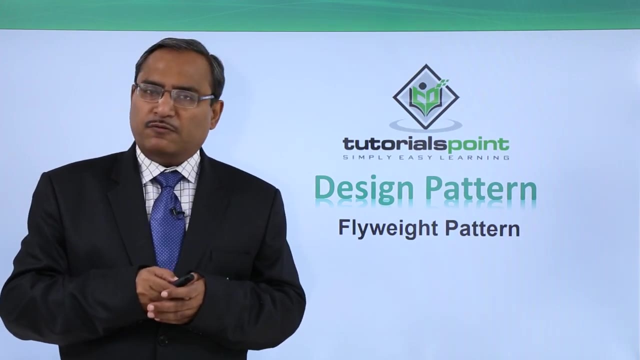 Flyweight design pattern. In case of flyweight design pattern, we shall always try to optimize the number of objects which are getting created so that we can have the lesser amount of memory during the runtime of the system and also to increase the performance of the system.